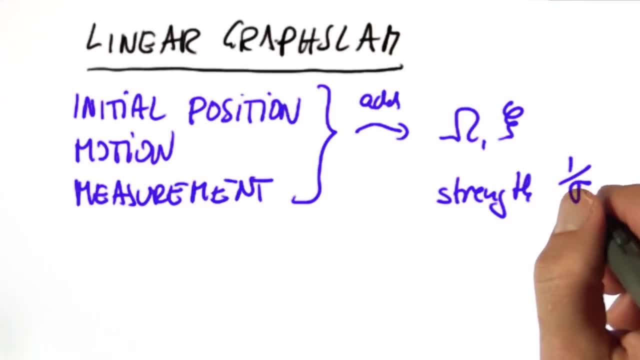 There's nothing else but 1 over sigma, the uncertainty in motion or in measurements. And then, when we're done with this, adding, we simply calculate this guy and out comes our best possible path and along with the map of all the landmarks. 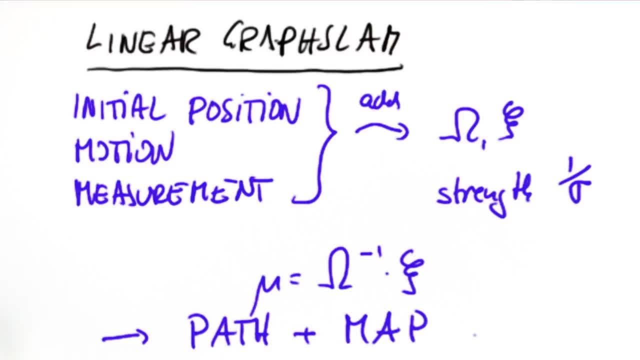 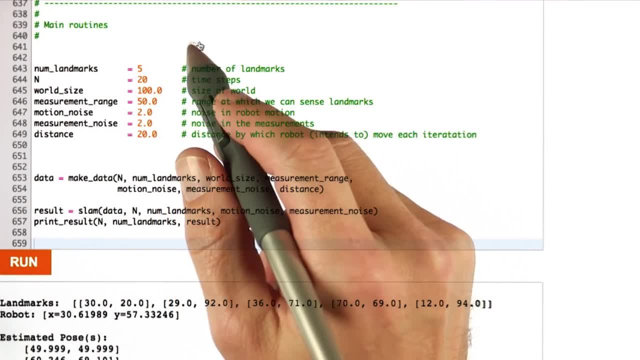 Isn't that something? Isn't that really cool? So let's dive in and have you program your own real robot example. This is a fairly complicated generalization of what we just saw. I'm giving you an environment where you can specify the number of landmarks that exist. 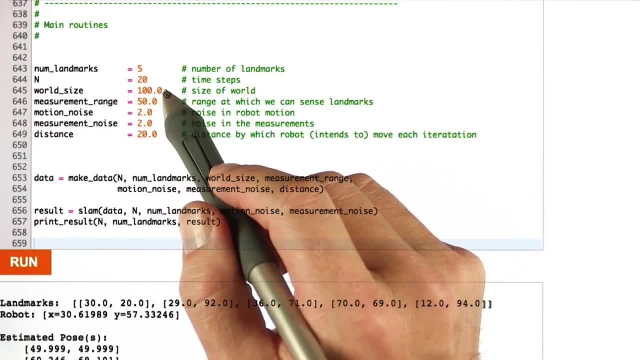 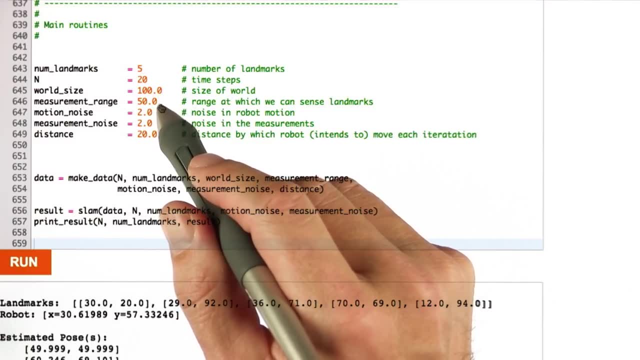 the number of time steps you want the robot to run. the world size, the measurement range: There's a range at which you want the robot to run? There's a range at which a robot might be able to see a landmark. If it's further away than this, it just won't see it. 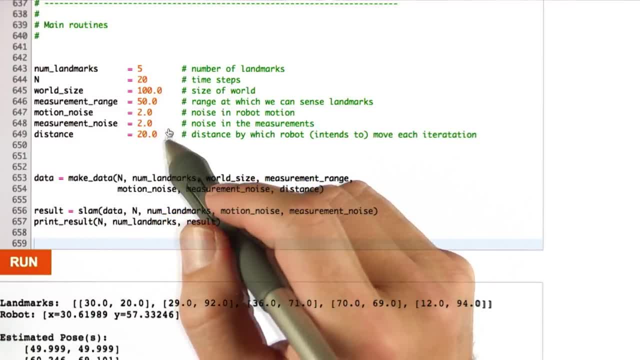 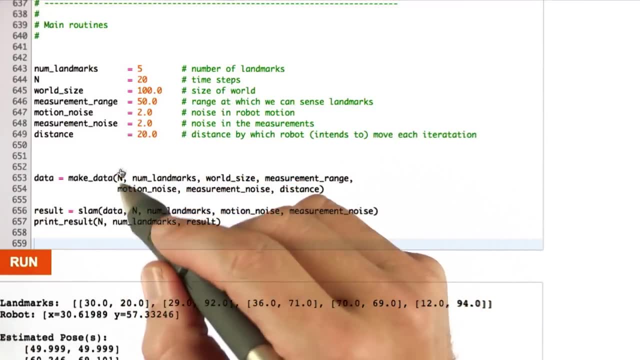 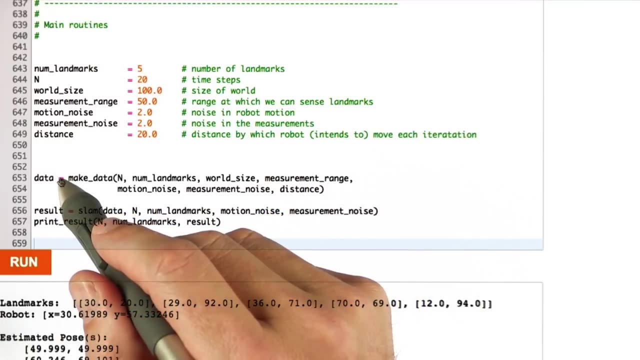 A motion noise, a measurement noise, and the distance parameter. The distance specifies how fast the robot moves in each step. And then I'm giving you a routine which makes the data. It takes all these parameters and outputs a data field that contains a sequence of motions. 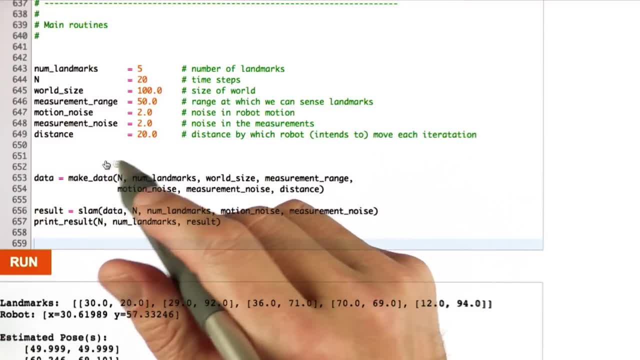 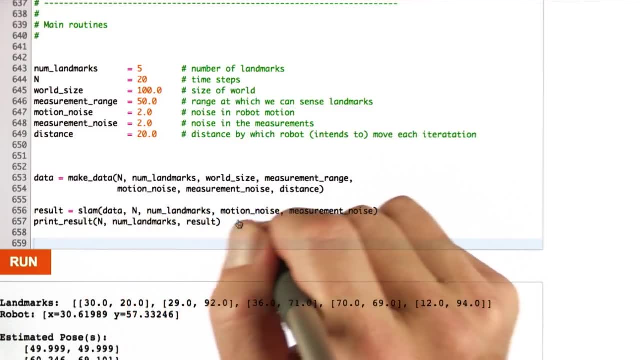 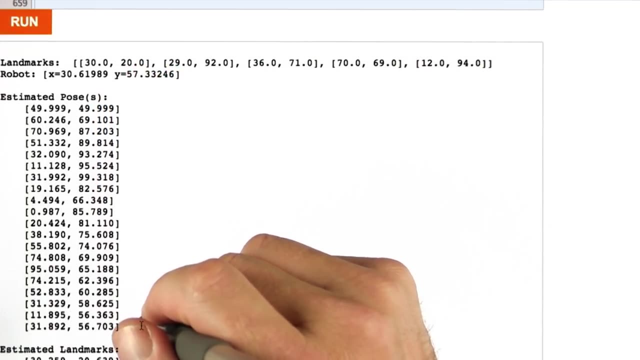 and a sequence of measurements. The code comments on the exact format of what data looks like. Now I want you to program the function SLAM that inputs the data and various important parameters and it outputs my result: a sequence of estimated poses, the robot path and estimated landmark positions. 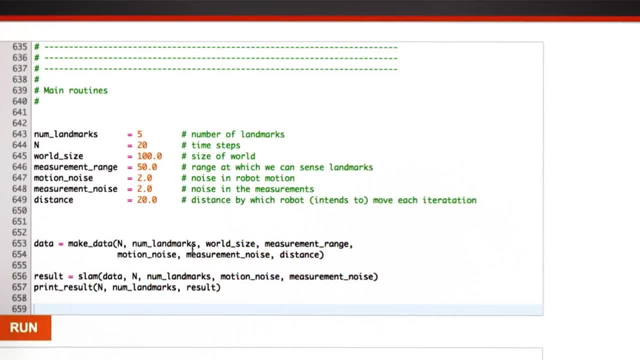 This is really challenging to program. It's based on the math. I just gave you The robot. coordinates are now x and y coordinates. The measurements are differences in x and y, so you have to duplicate things for x and things for y. I myself put them all into one big matrix. 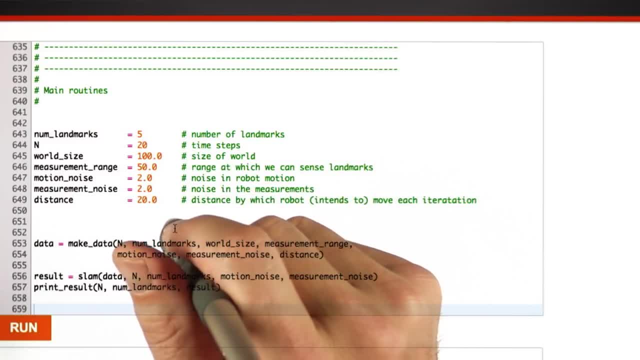 but you can have them in two separate matrices if you so wish. You have to apply everything we learned so far, including the weights of 1 over measurement noise and 1 over motion noise. These happen to be equivalent in this case, but they might be different. 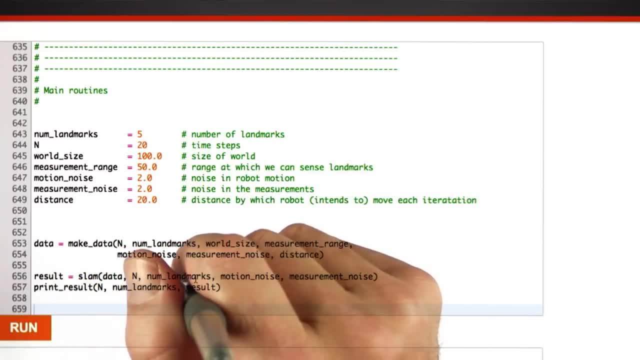 Then you have to run SLAM and return back to me a result data structure. I'm also supplying you with the print result routine so you can go in and see how the result has to look like. There's an example routine that doesn't work.